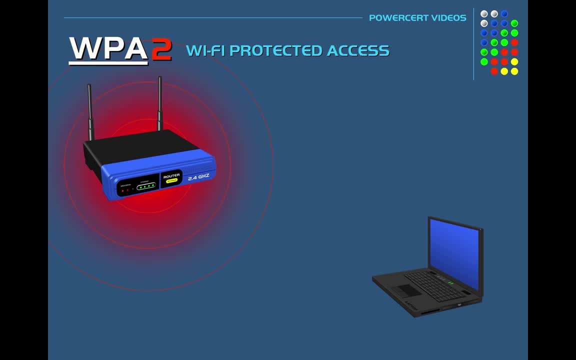 And that brings us to WPA2.. WPA2 was developed to provide even stronger security than WPA, And it doesn't support a flat OPC, so that's another thing that is likely to happen. this by requiring the use of a stronger encryption method, While WPA uses TKIP for encryption, which 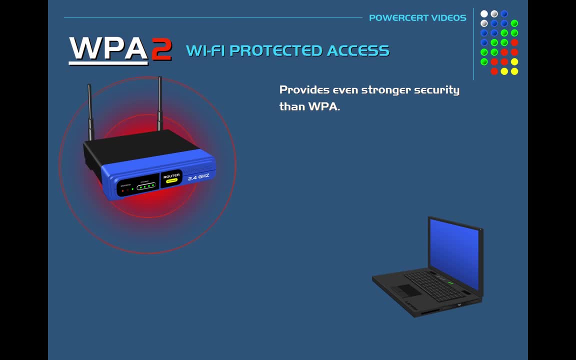 is known to have some limitations. WPA2 uses AES, which stands for Advanced Encryption Standard. AES uses a symmetric encryption algorithm which makes it strong enough to resist a brute force attack. In fact, AES is so secure that the US federal government has adopted it and is now using it. 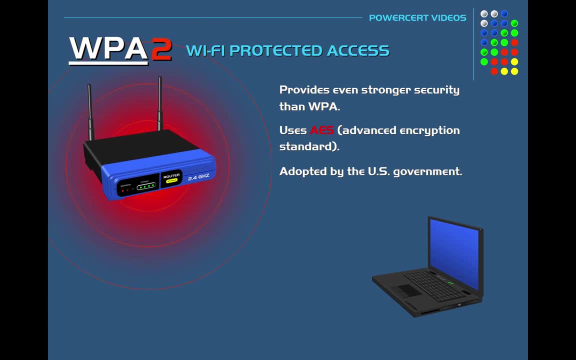 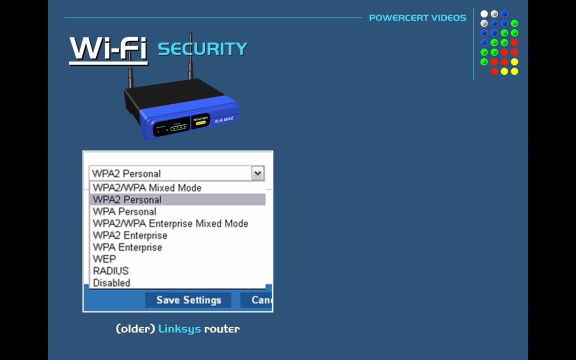 to encrypt sensitive government data. Now, when you log into the Wi-Fi routers configuration page and you go into the Wi-Fi security section, this is where you would find the different security protocols that you can choose from to protect your Wi-Fi network. So here is an example from 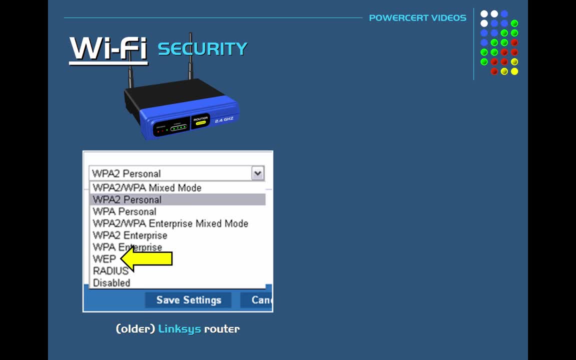 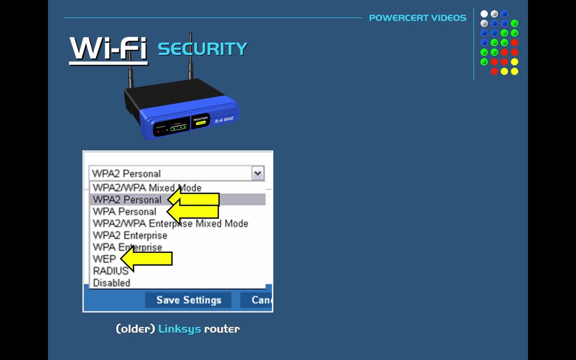 WPA2 are connected to each other, And here you can see the WEP and WPA2 are connected to each other: WPA and WPA2 protocols that we discussed. Now, as I said, this router is a few years old. 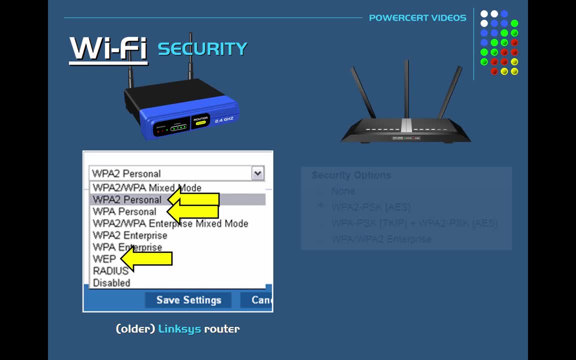 and it still has WEP as an option. However, newer routers like this one here won't even have WEP as an option, because WEP is weak and outdated and is no longer used, And thank God for that, because it was garbage. Now you will also notice that on both of these routers there's an option that has both. 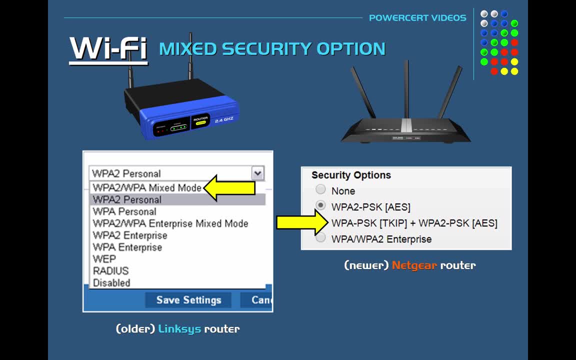 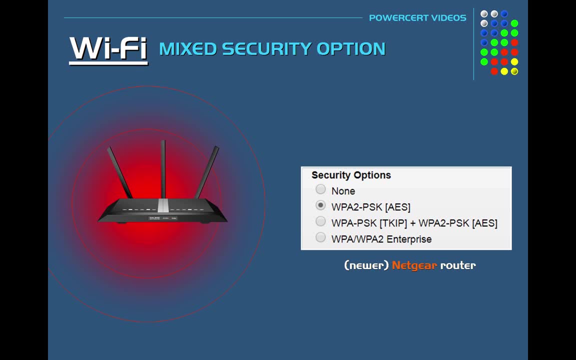 WPA and WPA2.. And this is a mixed security option. This option enables WPA and WPA2 at the same time, So it'll use both TKIP and AES security. Now, the reason for this option is for compatibility purposes, Because some older devices, like prior to 2006, may not be compatible with using AES. 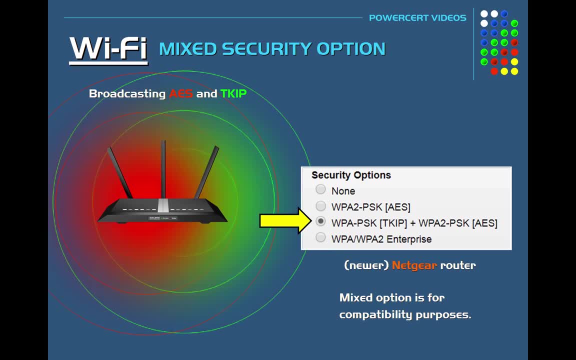 encryption that's used with WPA2. And so these older devices may not be compatible with using AES. Now some devices will connect to the older WPA protocol, But at the same time, modern devices will connect to WPA2.. Now some people might ask: why not just choose the mixed option all the time? 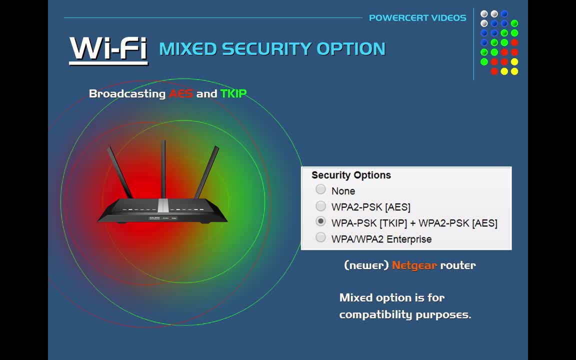 since it's the most compatible with all devices. Well, you can do this, but the problem is is that, in addition to using AES, it's also using TKIP, And since TKIP is not as strong as AES, you're leaving your network more vulnerable to a breach, And so you can't use AES to protect your network. 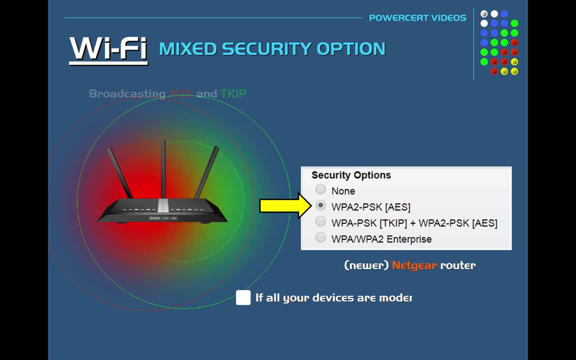 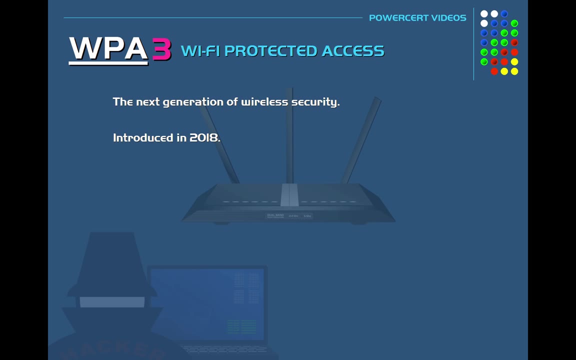 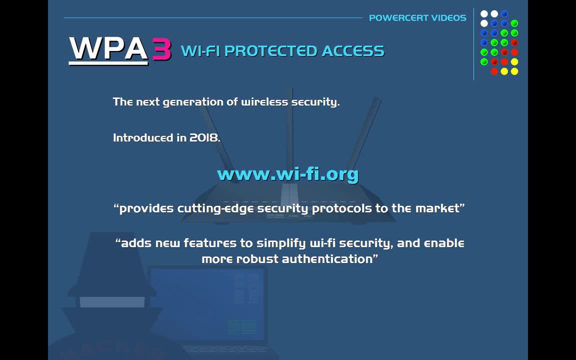 Wi-Fi security and enable more robust authentication, And it will receive increased protections from password guessing attempts. Now, WPA3 won't be available on every Wi-Fi router that you purchase today, because it was just introduced last year. However, you will start. 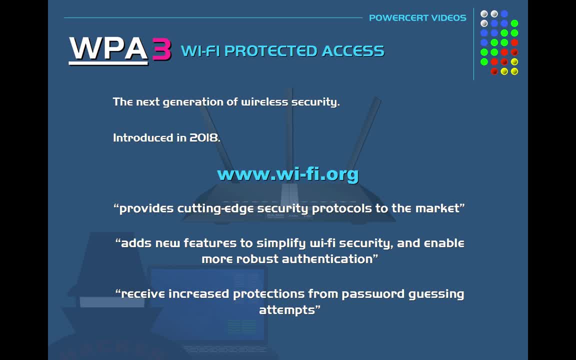 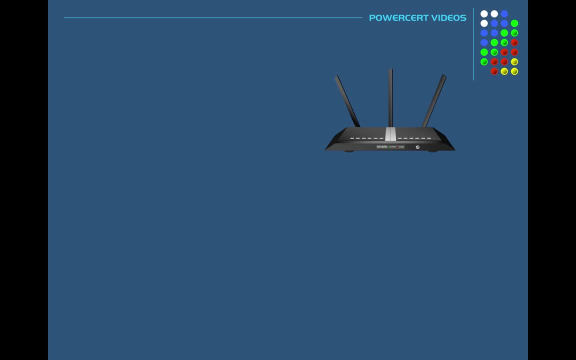 to see it more and more on Wi-Fi products in the next few months Now. so far, we discussed a few password-protected security protocols, but there is a lot of information about how to use WPA3.. There is another wireless security method that doesn't require you to type in a password, And 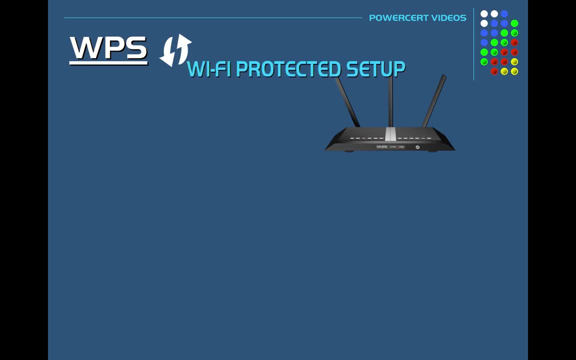 this method is called WPS. WPS stands for Wi-Fi Protected Setup, And WPS was designed for people who know little about wireless networks to make it as easy as possible for their devices to join a wireless network. So here is a WPS configuration page for our router And there are a couple of 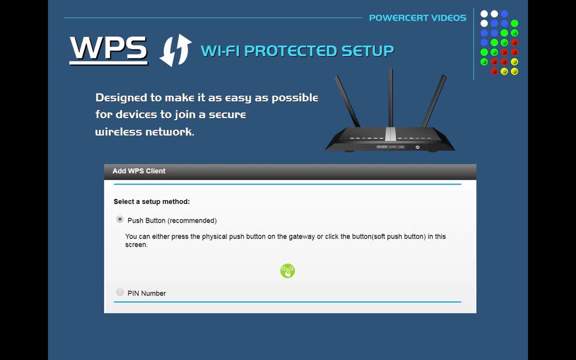 different methods that are used to configure WPA3.. One of them is the WPS configuration page, But by far the most common method is the push-button method. So with this method you would just press a couple of buttons and then you'll be connected. So, for example, most routers today will.